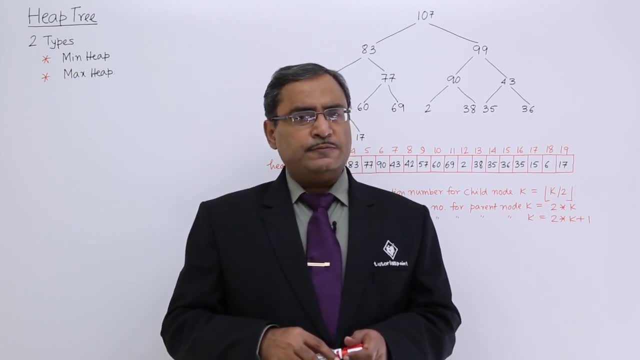 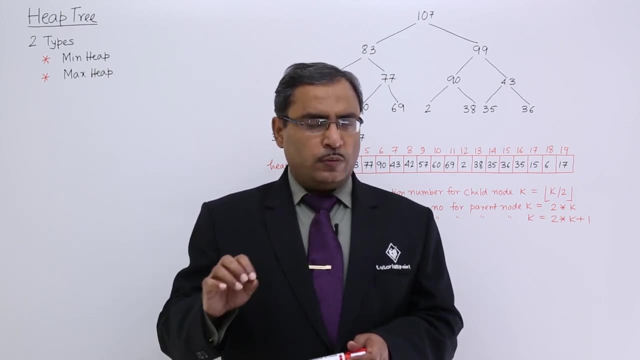 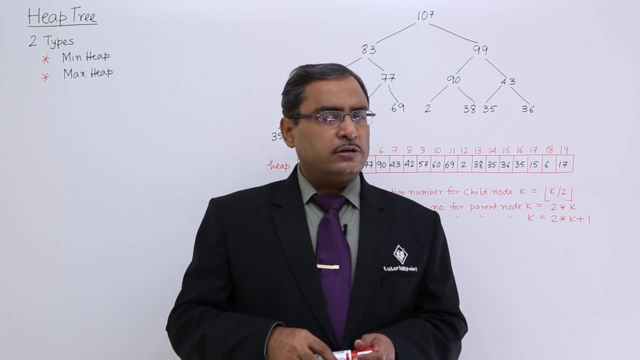 possible. but if it is not there, in that case, from the extreme left child to the last child, whatever it is having on that very last level should be continuous. There should not be any child missing. That is known as a complete binary tree. If it is not there, 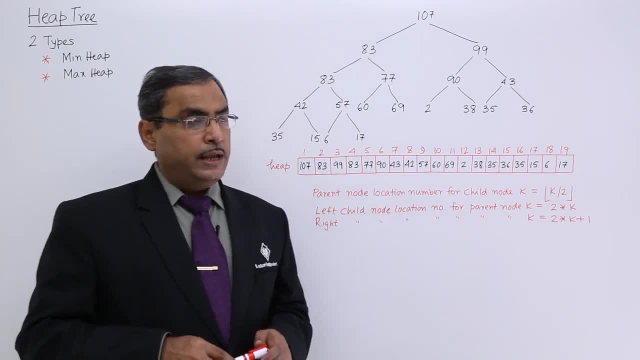 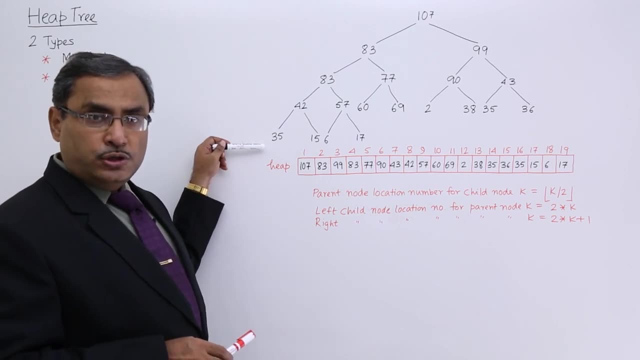 it is not clear to us. let us see this particular binary tree. It is a complete binary tree, So it is having level 0, level 1,, level 2, level 3,, level 4.. So up to the last but one. level. that means level 0, level 1,, level 2 and level 3, we are having maximum number of nodes per level, So the first level, level 0, we are having only one node. level 1, 2. 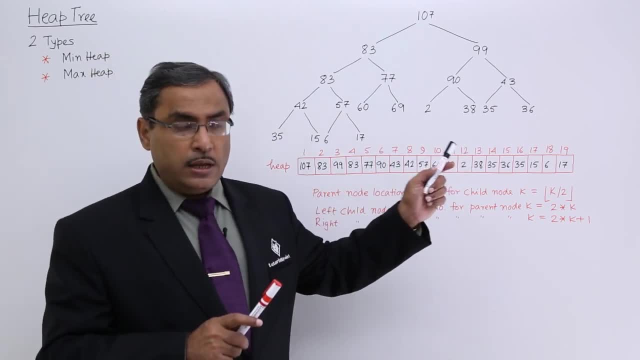 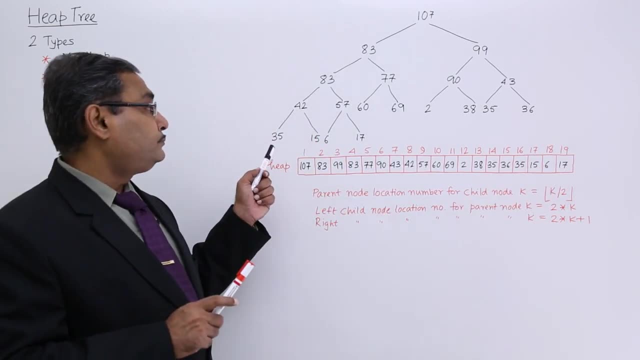 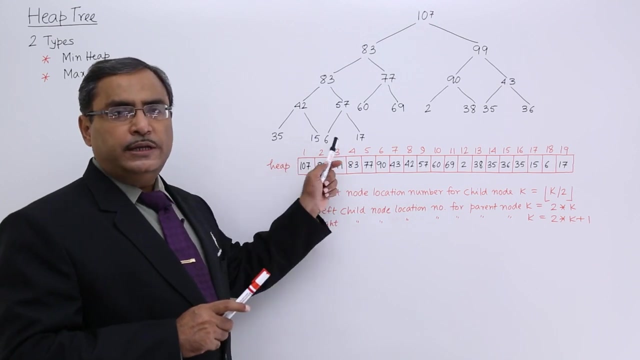 nodes: level 2, 4 nodes, level 3, 8 nodes, but the last level can have maximum number of nodes. but if they are not there, then from the extreme left child to the last child, whatever it is having, all the child must be there. There should not be any missing. 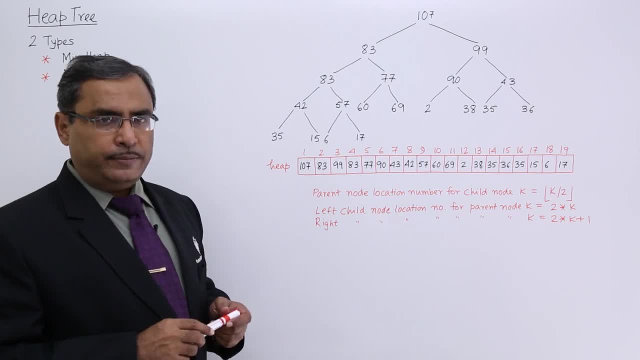 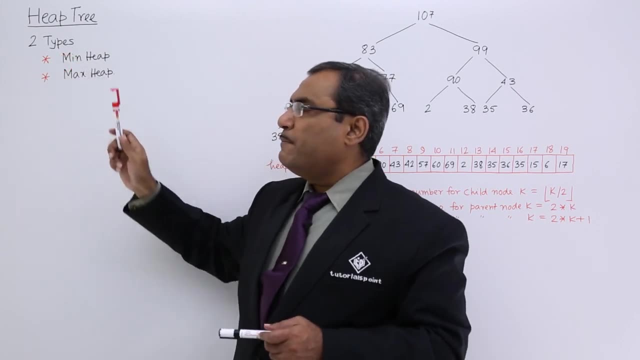 child and that is known as a complete binary tree. So that is, the complete binary tree, is the first property and it will be of two types. One is a min heap, another one is a max heap. Max heap means max heap means, if you consider, 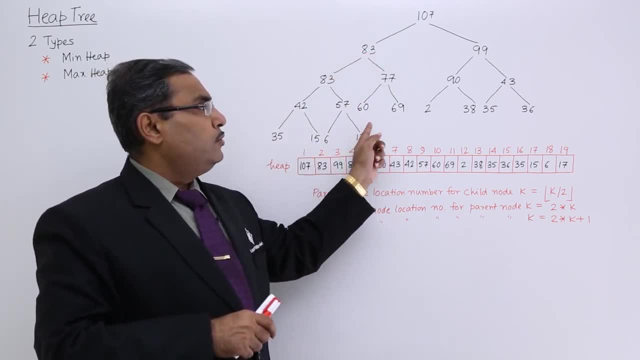 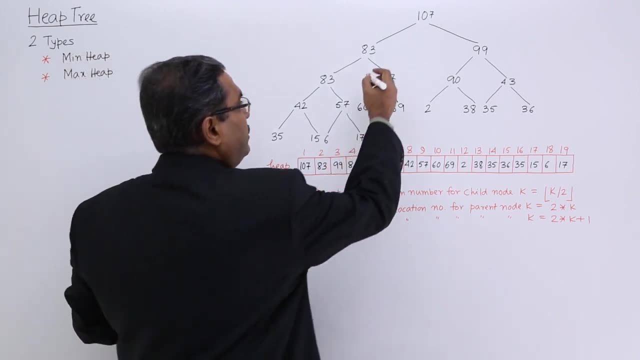 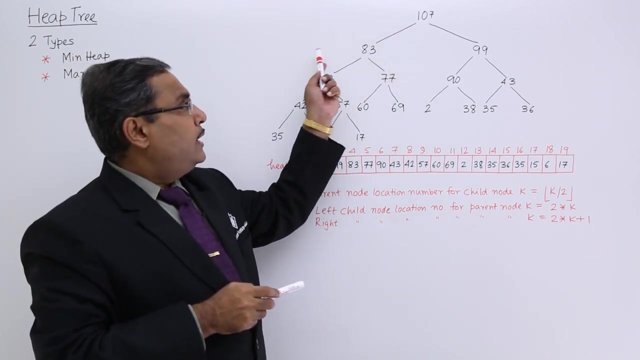 any node, Then all the successors of this particular node will be either lesser than this or equal to this, So that is known as a max heap. That means a tree. whatever I have drawn here is nothing but a max heap. Just consider 107.. It is a maximum number and all the successors 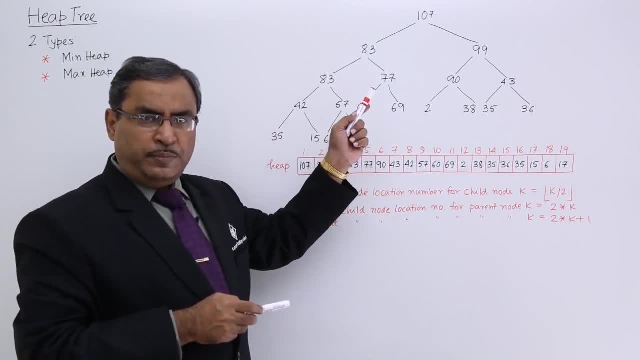 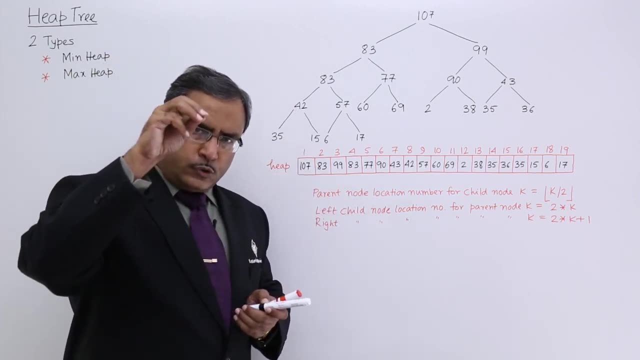 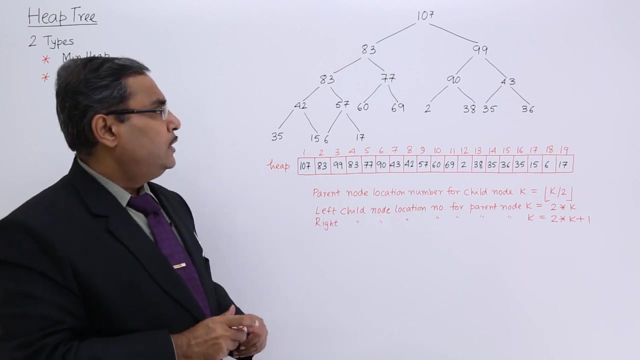 whatever it is having. either they are equal to 107 or lesser than that. In the min heap just the reverse thing will take less. That means any node will be less than or equal to the nodes in its successor. So that is known as the min heap. So this 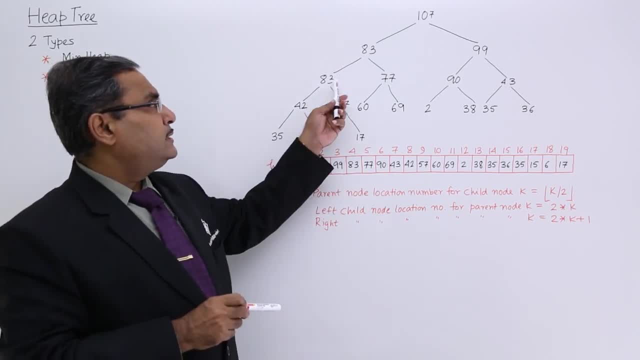 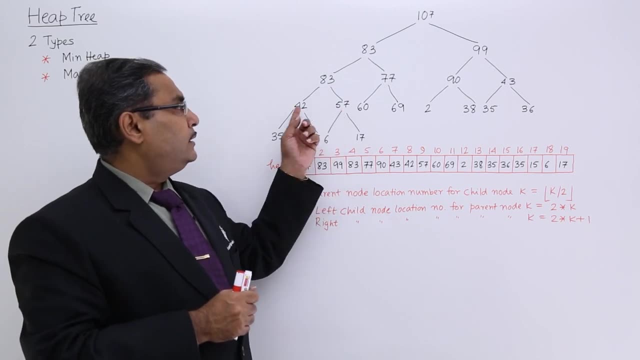 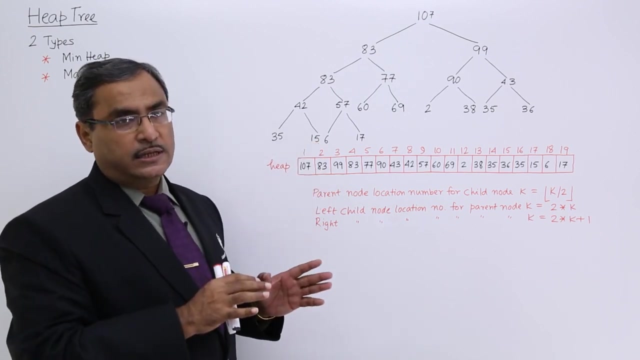 is my max heap. Here you see, the numbers have got repeated. The numbers have got repeated and here you see, the right child is greater than the left child, and sometimes the left child can be also greater than the right child. So there is no such restrictions, are there? 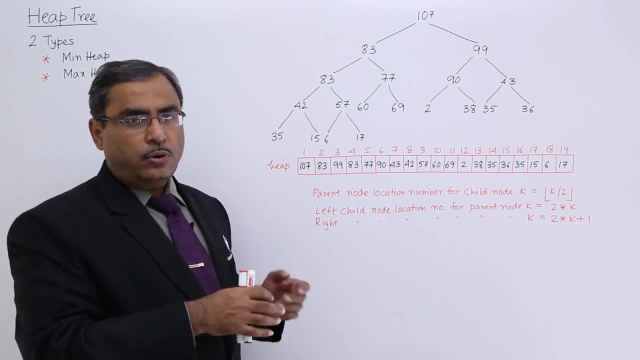 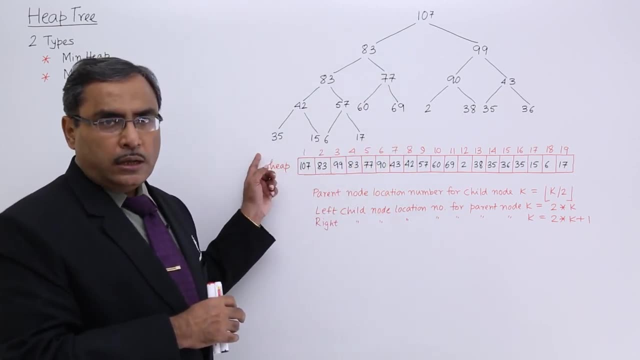 Numbers can repeat. Right child can be lesser than or equal to or greater than the right child. So left child will be greater than, less than or equal to the right child. So this is my. this is known as the hip tree. So two properties I have explained and complete. 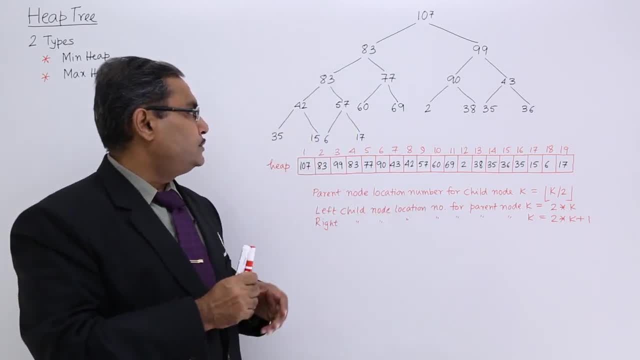 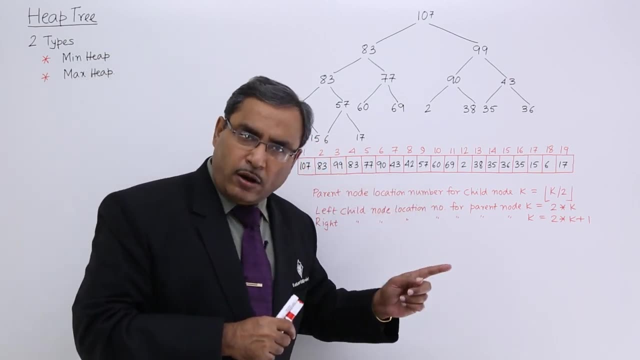 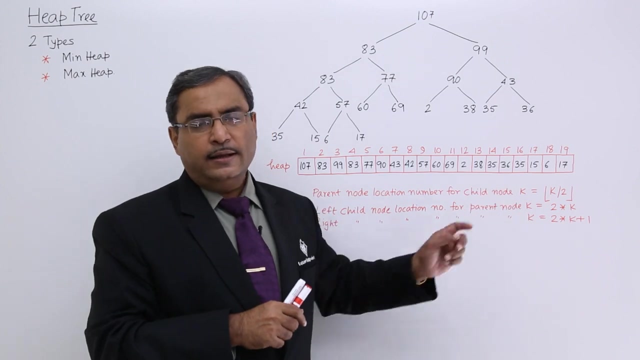 binary tree is another extra property. Now see, as it is a complete binary tree, we can represent this hip tree in the form of an array, because, as it is a complete binary tree, so if you represent this particular tree in the form of an array, then there will 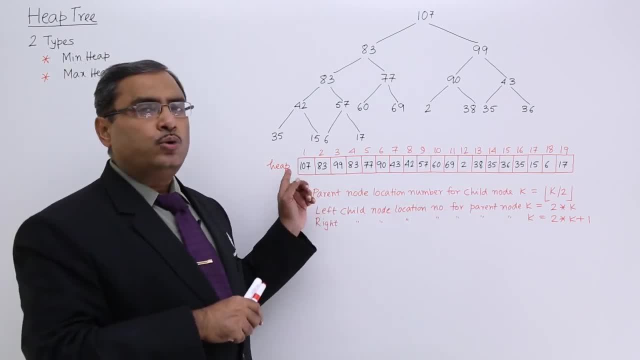 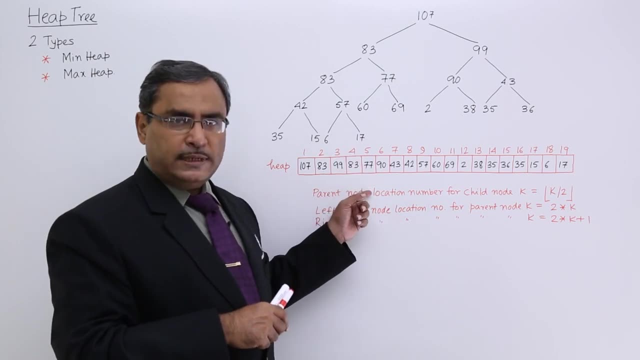 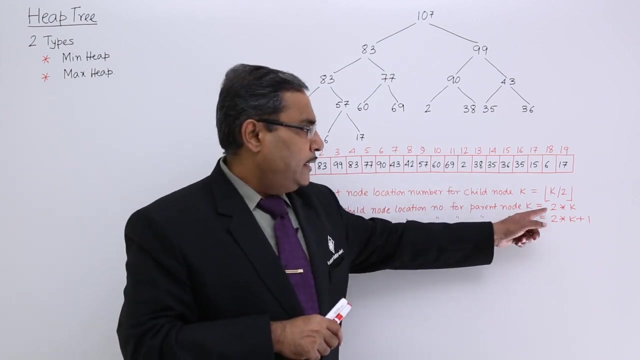 be. no blank spaces are there in the array. So the array will be totally dense. And you know that whenever one array will get represented, whenever one tree will get represented in the form of an array, then the kth node left child will be at the place 2, star k and right. 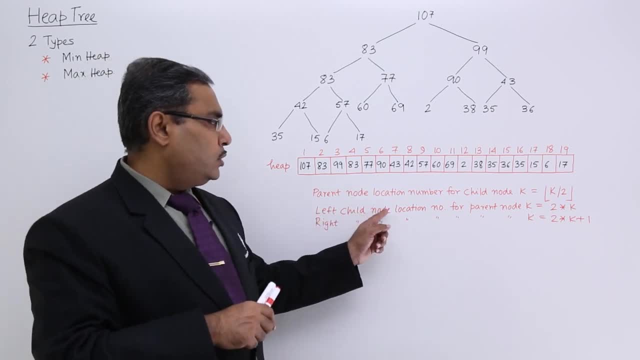 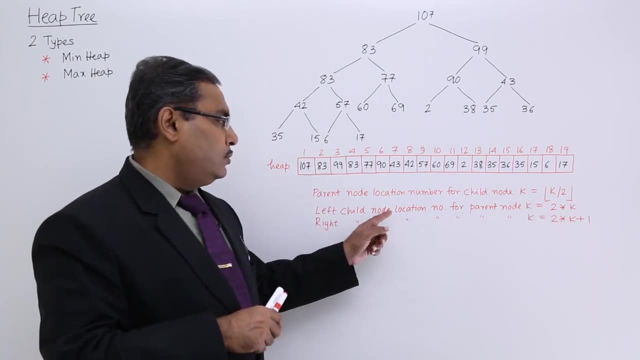 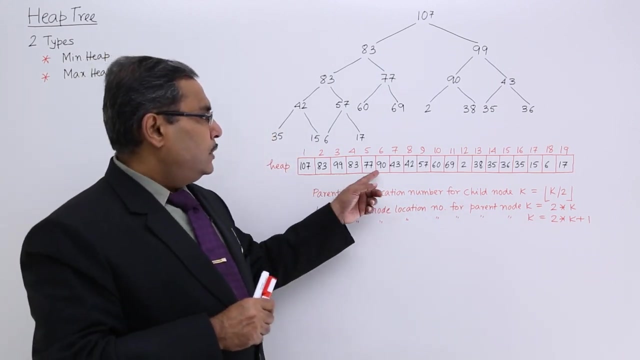 child will be at the place: 2 star k plus 1.. Left child node number: node location number for parent node k is 2 star k and right child node location number for parent node k is equal to 2 star k plus 1.. Let me explain that one Now. let us suppose say I am talking. 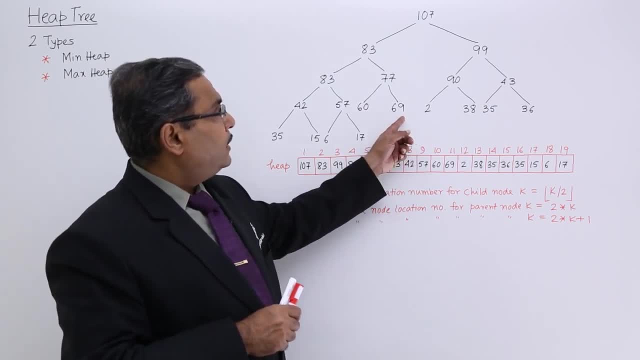 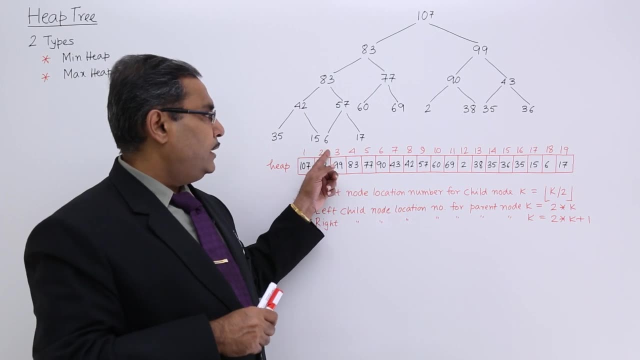 about say 99,, 99. So 99 is which one? 99 is this one. Its left child is 90, right child is 43. So 99 is at the location number 3.. So at the 6th location I am getting 90,. 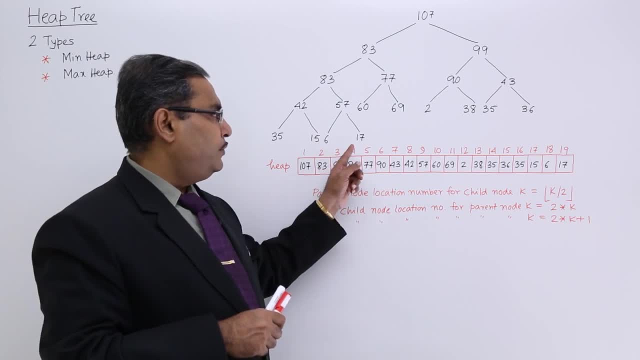 at the 7th location I am getting 43.. So how to get 6 from 3? That is, 2 into 3.. How to get 7 from 3? 2 into 3 plus 1.. So this is my kth node. So this is the kth node. So 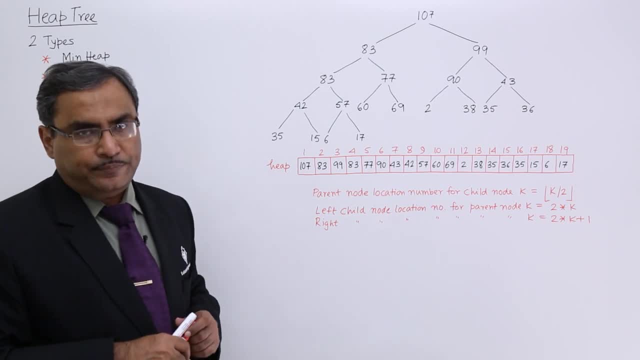 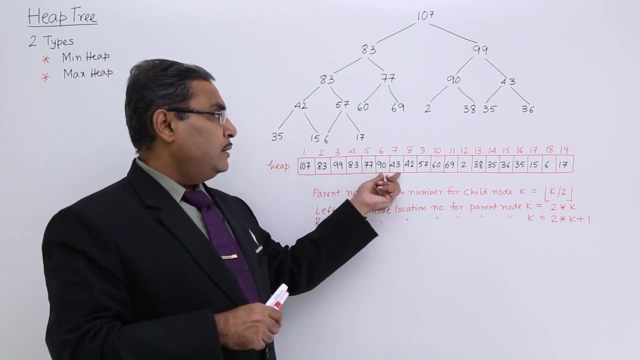 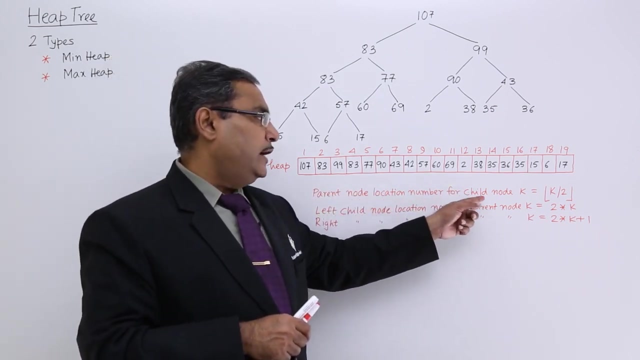 1. in this way, if you go on checking you will get the same. now you see 90 and 43. they are having the parent 99. So location number 6 and 7 will have the parent at location number 3. that means parent node. location number for child node k is equal to k by 2 floor of that. 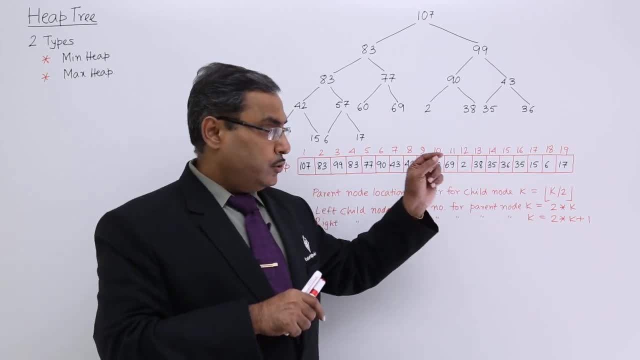 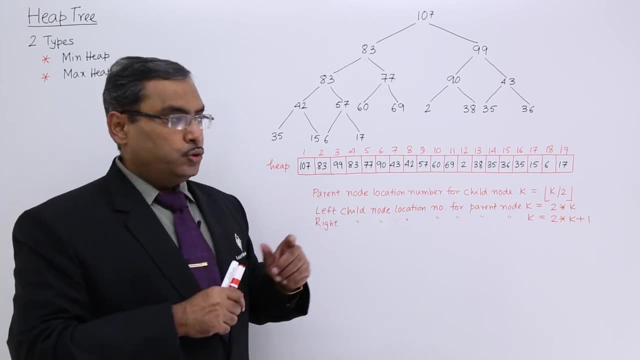 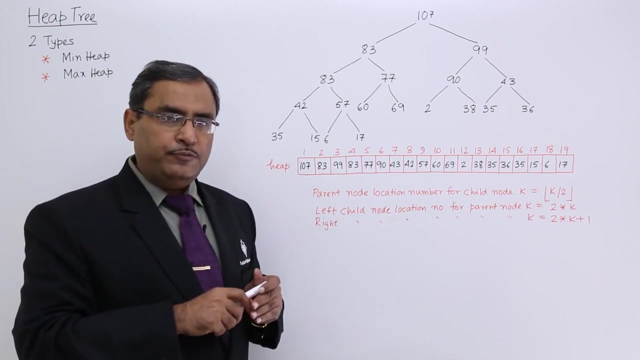 k by 2 floor of that. it is not third bracket, it is a floor. So k by 2, floor of that will give you the parent nodes address in the array. So this concepts will be required in our next classes. and in the next class we shall discuss the insertion of a heap tree. So 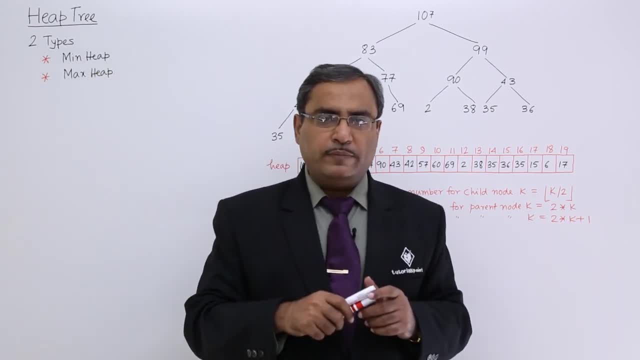 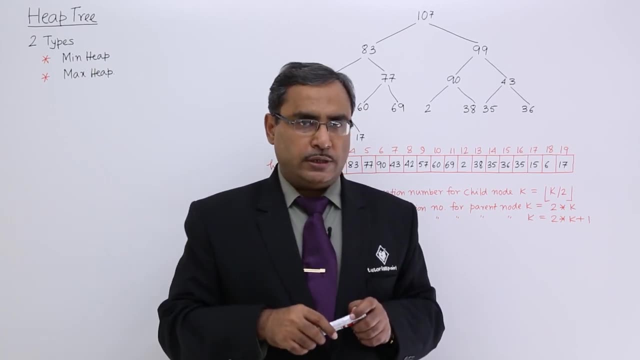 we shall carry out insertion operation on a heap tree. So how to perform the insertion, that will be the topic in the next video. Please watch all those videos because they will be in the continuation. Thanks for watching this one.